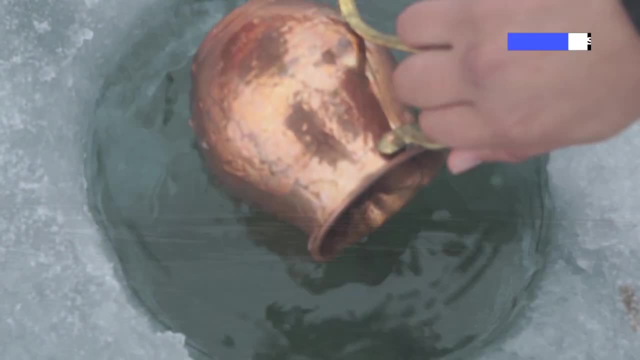 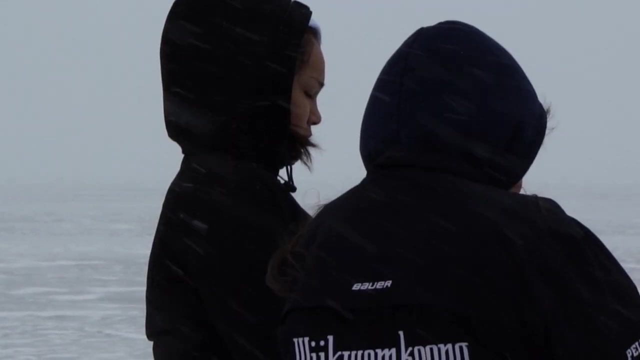 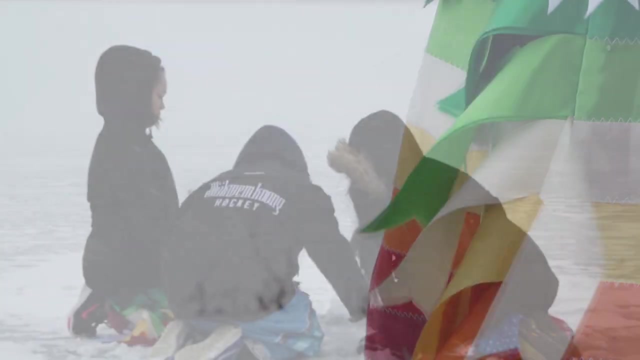 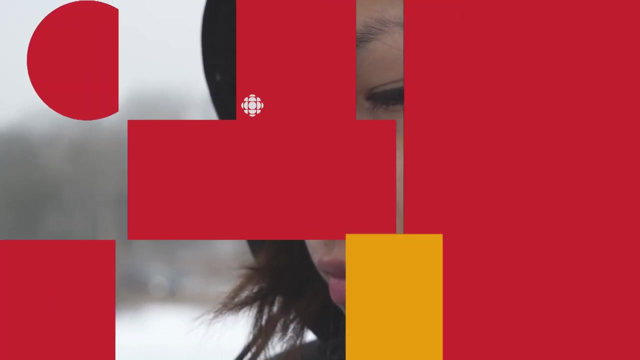 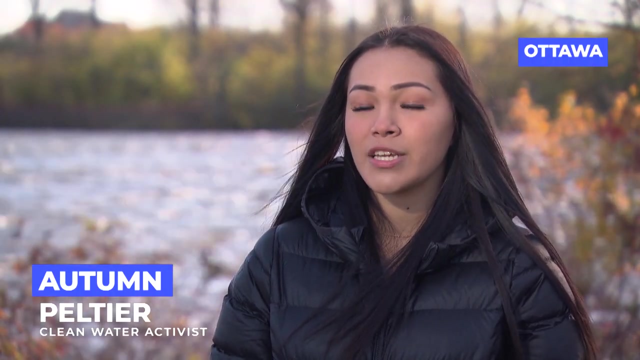 We go out and pray for the water because the water is sick and it's contaminated and we basically just do the water ceremony to pray for it, for hopefully one day that the water's clean. My name is Autumn Pelche. I'm the Chief Water Commissioner for Anishinaabek Nation. 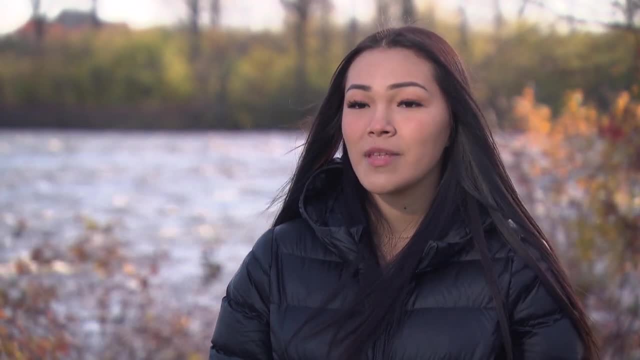 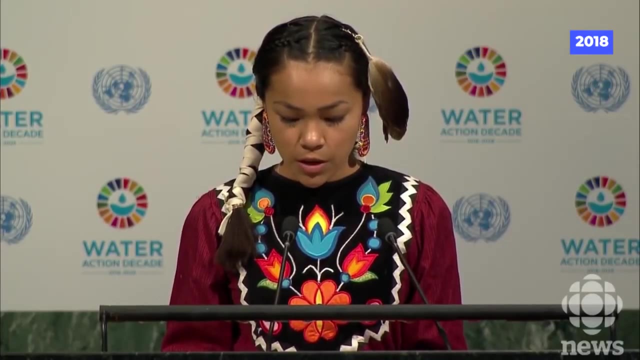 I'm 16 years old, I'm from Manitoulin Island and I'm currently living in Ottawa. I'm doing this work as we can't just pray anymore. We must do something, and we need to do it now. Water is a basic human right. Everyone deserves access to clean drinking water, no matter what. 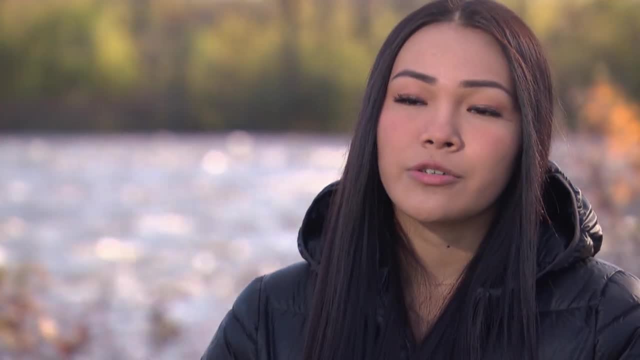 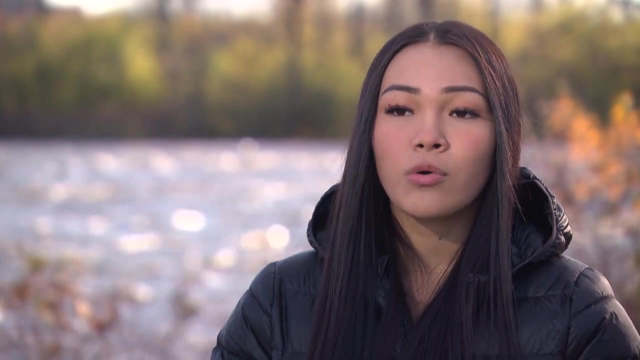 our race or color is, or how rich or poor we are. When I was eight years old, I was attending a water ceremony in a First Nations community. I asked my mom to go to the washroom and all over the wall said: don't drink the water, not for consumption. boil water advisory. 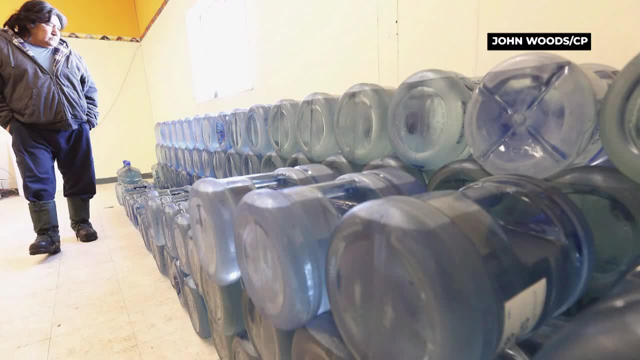 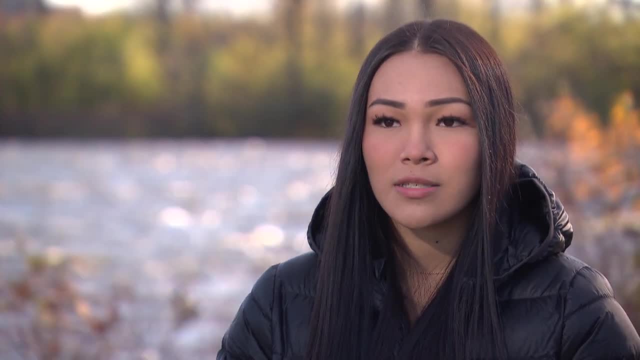 And we had to use hand sanitizer after using the washroom, and I was very confused as to why it was like that. So I asked my mom: what does all of this mean? Why can't we drink the water? Why can't we wash our hands? And then she explained to me what all of it meant: what a boil water? 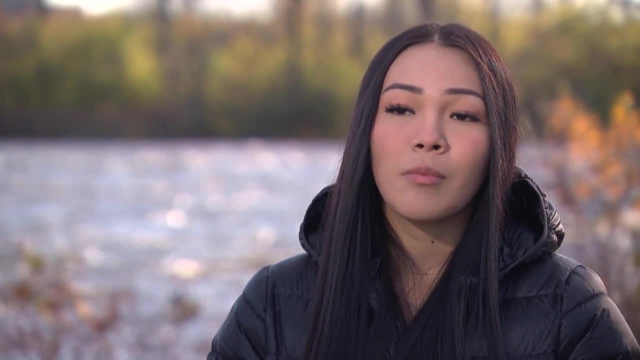 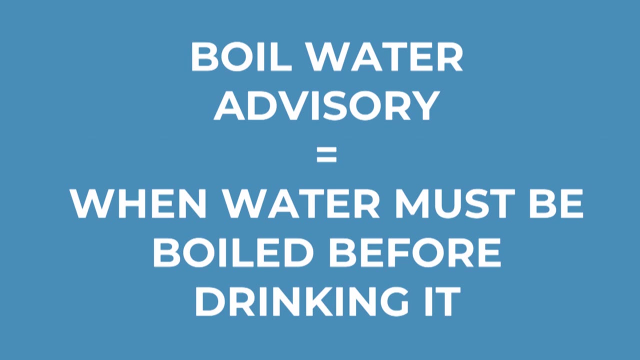 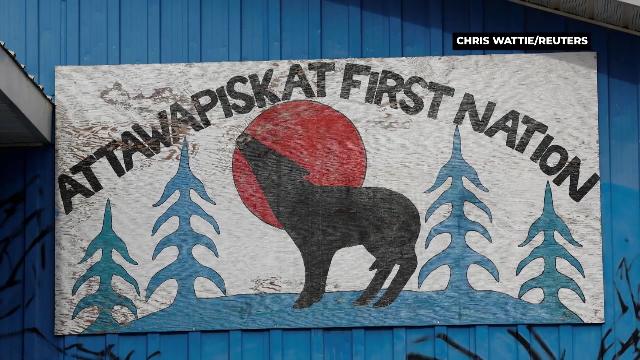 water advisory was and that the community that we were in has been on a boil water advisory for over 20 years. I visited a First Nations community, I think, last summer and it's Attawapiskat First Nation. They're a northern community in Ontario and I had a chance to speak with the youth there. 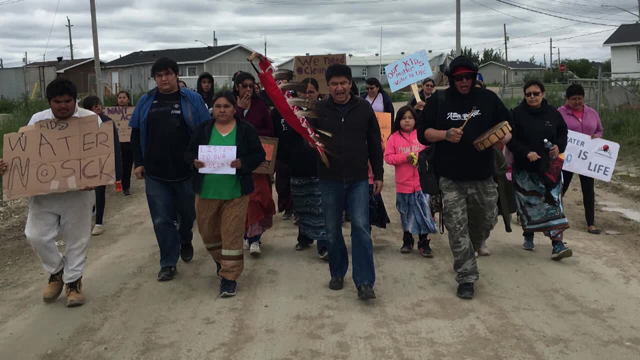 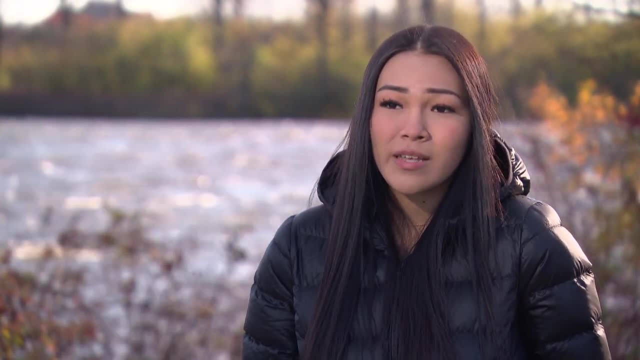 and, honestly, some of the things they had to say were really. they were heartbreaking. they were really sad. One of the kids said to me that she feels bad that her grandparents, who are both over 70, have to walk every day Two kilometers with buckets of water to get their water from a well. 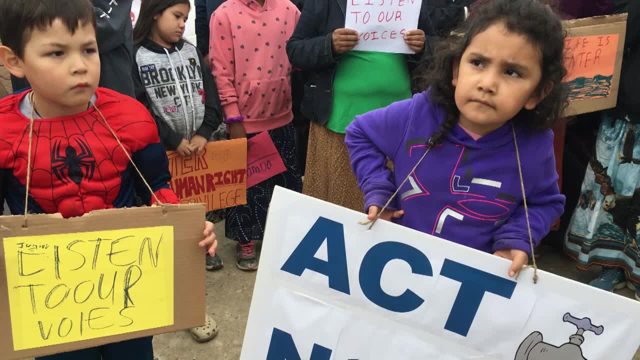 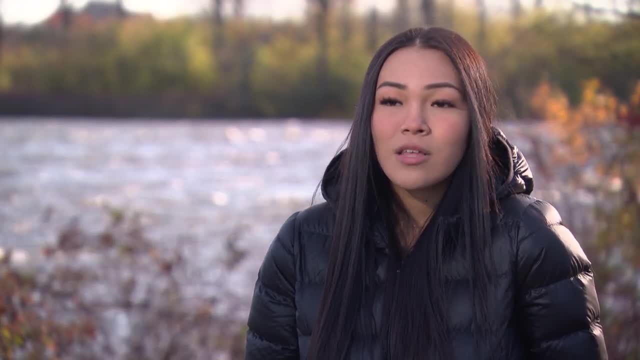 that everyone in the community has to share And, honestly, that's terrible. I went there and you wouldn't even think that you're in Canada. They're living like I said: they're living in third world conditions and we're in a first world country. It should not be like.